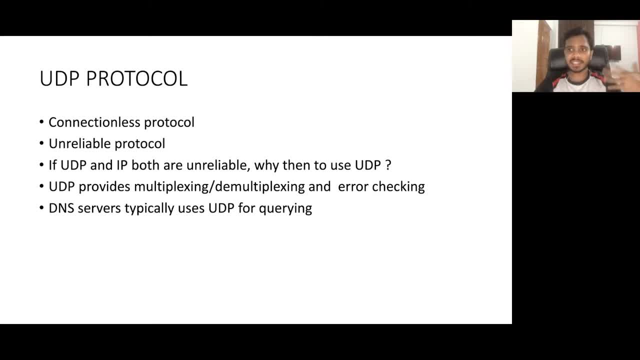 it's not guaranteed by the udp protocol. it tries its best but it will never guarantee you the same. now you will think that if udp and ip, both are unreliable. so i have discussed about a difference between uh ip protocol and transport layer, like transport layer protocol. in one of my videos i 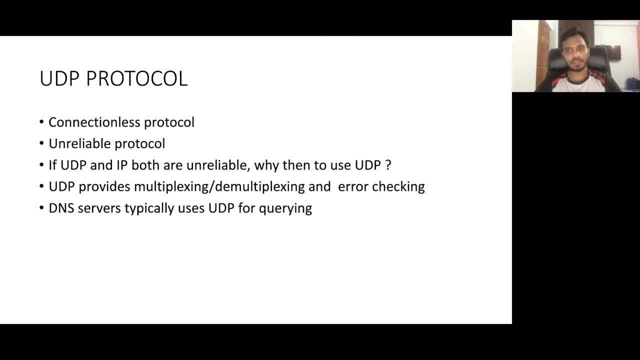 think two videos before, before this. now you can think that of course ip protocol is also unreliable protocol and ip protocol is a part of network layer. now you will think that if udp and ip protocol both are unreliable, then why then to use udp? why directly? and why directly? we cannot. 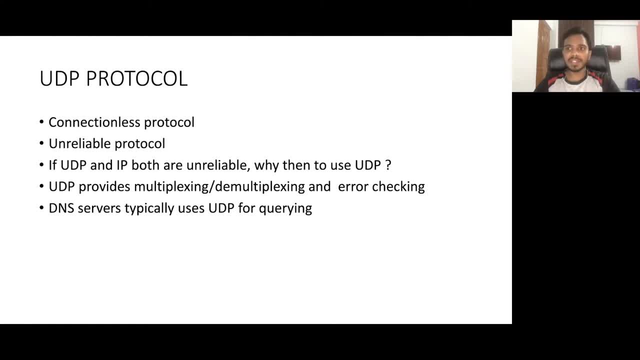 so why can't we directly use the ib protocol? why even to use the udp protocol? so the reason is that udp does provide some benefits, since udp is a part of transport layer. it does provide multiplexing and demultiplexing that we have seen in the last video, and also it provides 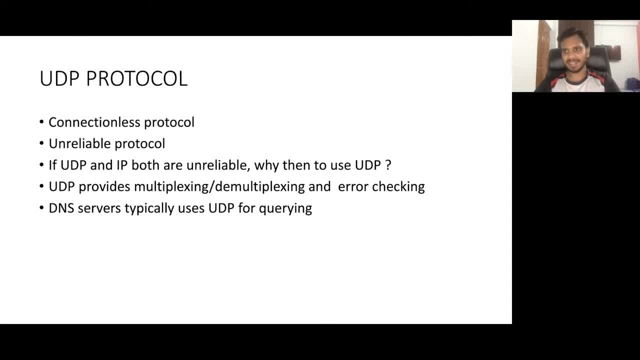 some error checking. so other than these two, it does not provide anything. so tcpu will see it provides a lot of features, but udp is kind of so in in terms of reliability, if you see it provides nothing, i mean. so it's just what it provides is just these two: multiplexing, demultiplexing. 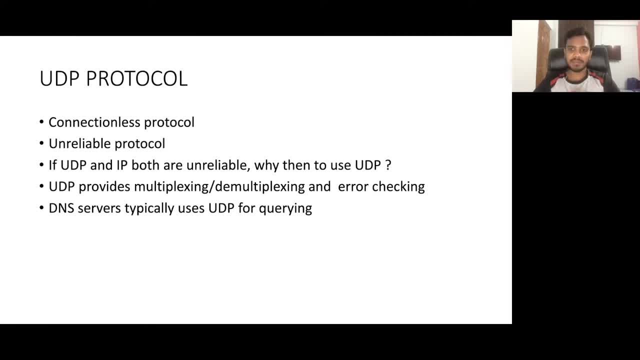 plus error checking. and now you will think that, okay, why, why not implement the same thing in the ib protocol, right? i mean, that will again make the overall networking layers right. it will make it complex. so that's the reason we have four or five layers, right, uh, in tcp, ip, or, or we have the os, ospn. 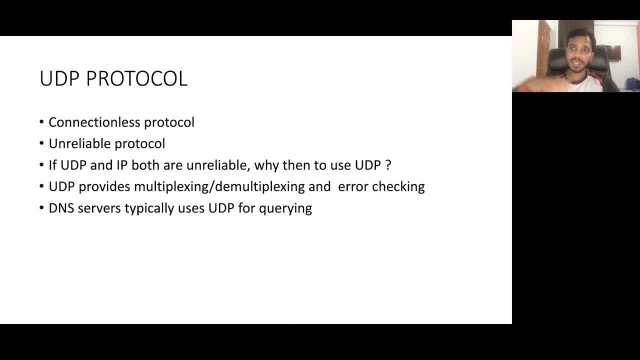 model right to make the. uh, i mean the, i mean to make computer working easy to understand. now, if you put the multiplexing, demultiplexing, also in the ip protocol, then it will become a bit messy. also, one example of service that uses a udp for querying is dns. like dns typically, it will use. 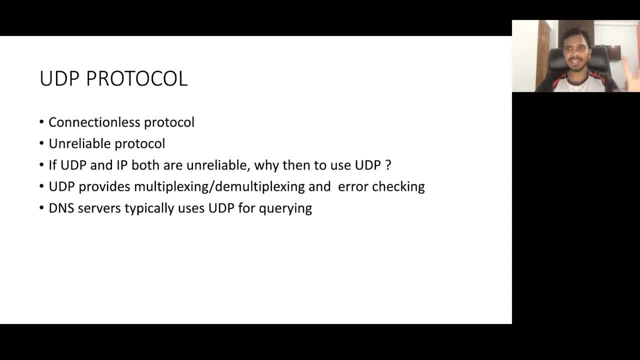 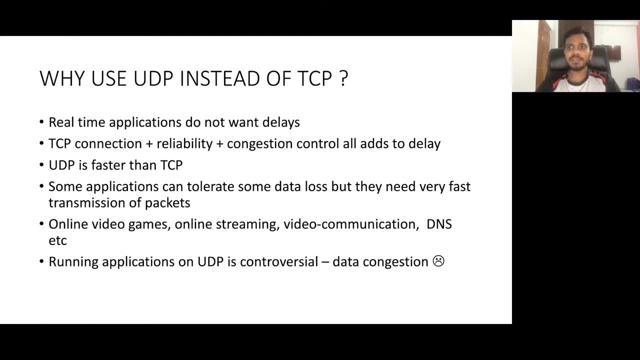 udp protocol for querying the dns servers and we have seen this in uh when we, when i was discussing about uh dns in one of my videos. okay, now i have explained you why to use udp over ip protocol. i mean why we cannot integrate multiplexing, demultiplexing, into the iv protocol itself. 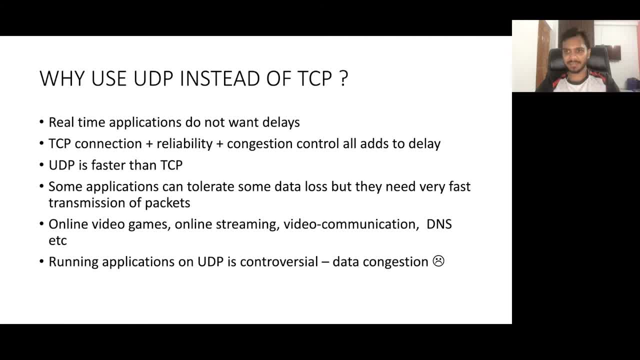 but the next question is again: why use udp instead of tcp? so we know that tcp is a reliable protocol. tcp is the connection oriented protocol. so tcp provides reliability right, which is very important. you do not want like, if you send some data you do not, i mean you. you do want guarantee right most. 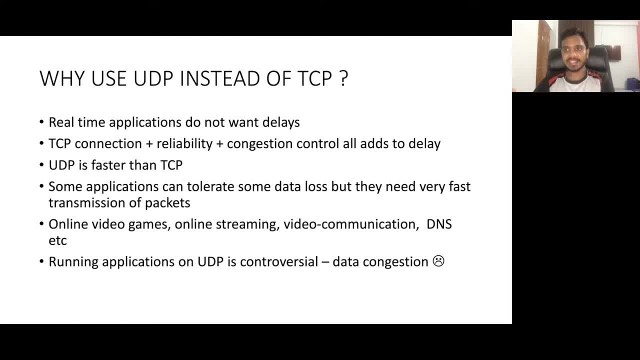 of the time that that data should reach the destination. and this tcp gives you that. and why do you use udp? right? you will think again. you will, of course, have a question in your model mind. so the reason is: i've explained the reason why sometimes udp is used, and already we have. 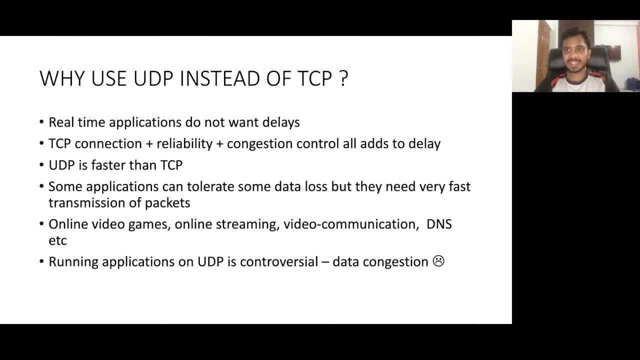 seen that in dns, udp is used, so of course there will be some reason that dns is using udp over tcp, right? the reason is that, uh, real-time applications do not want delays, okay. so real-time applications examples are: like: you are playing some online games, okay. uh, you are doing a like. 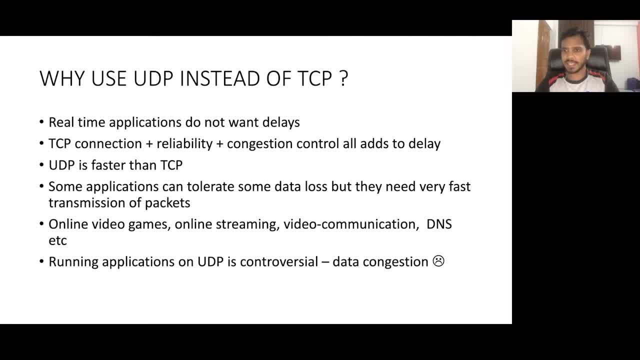 video conference, right, or like over zoom or skype or any other, uh, like such services. now, what happens to tcp connection? is this in this real-time applications? now, of course, tcp is connection oriented, so for tcp connection the client has to first initiate a connection to the server, and that 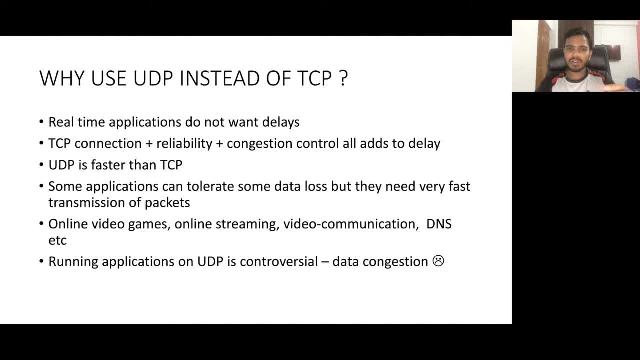 will add, to delay overall delay. plus, there are a lot of like. there are a lot of things that goes in the background, like for tcp to make the overall process reliable. so we will go into some details in the next videos. but there is there is a lot of things that goes in the background and all of 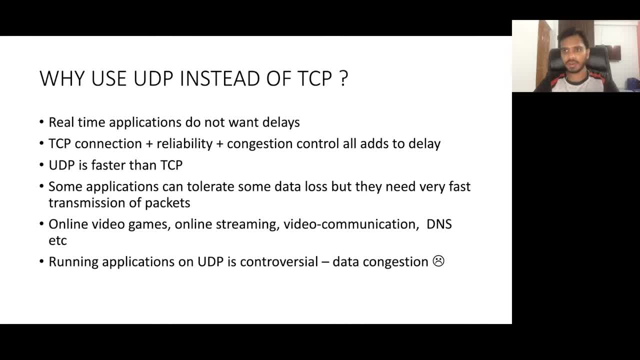 those do add to a a bit of delay to the overall connection. so that's one of the things that we are going to talk about in the next video. so let's talk about tcp communication. udp is faster than tcp. the reason is that because, because of the connection oriented nature of tcp, it takes it. 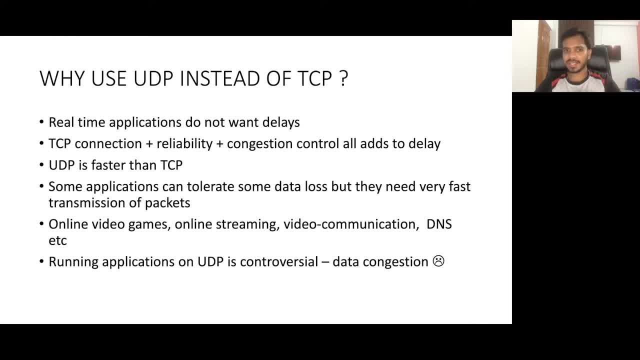 uh, i mean more time than udb. root of all or some applications can tolerate some data loss. so there are these applications. this real-time application can tolerate some data loss, but they need very fast transmission of packets or they need very fast transmission of the data. that's why they use. 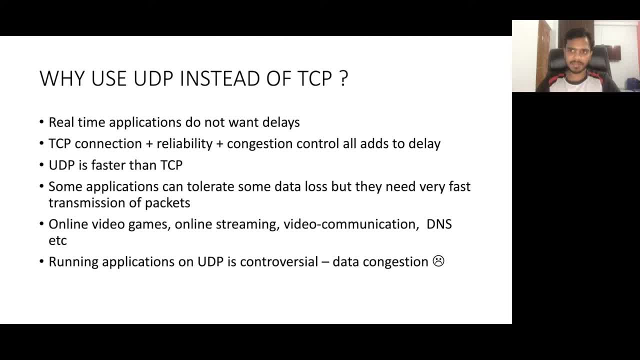 udp. so for them, okay, it's fine. okay, if some of the packets do not reach the destination, it's fine for the communication to be very fast. these real-time applications, for example, online video games, online streaming video communication and dns for in these online video games, online streaming video. 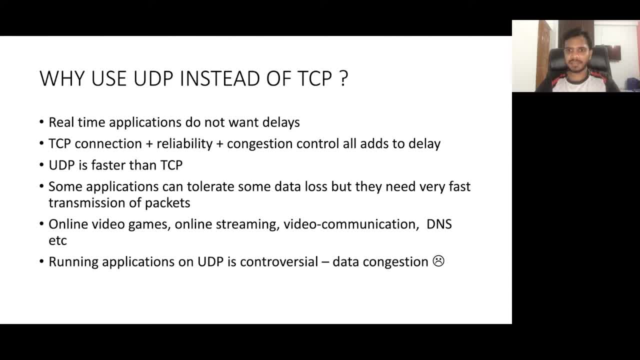 communication. i mean you may adjust with some data loss, like if the quality goes a bit- i mean low- sometimes, it's fine for you, but it should be fast. i mean it should be very fast. you do not want delays in the communication in this. so now take example of dns. so whenever you visit a website on 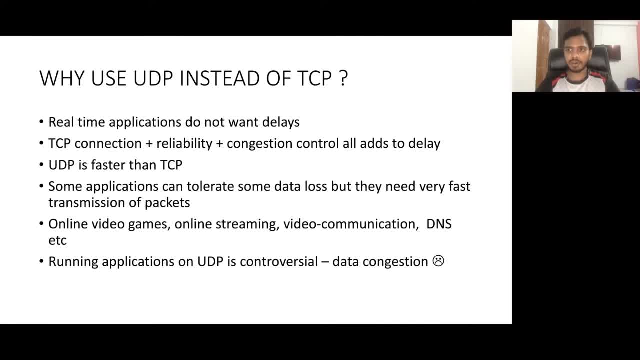 your browser. a dns dns query is uh used for resources like dns query and dns query is used for solving the website to ip address. now what will happen if dns is i'm a dns user tcp. so every dns query will take a lot of time and that will add to the overall like experience on your browser right. 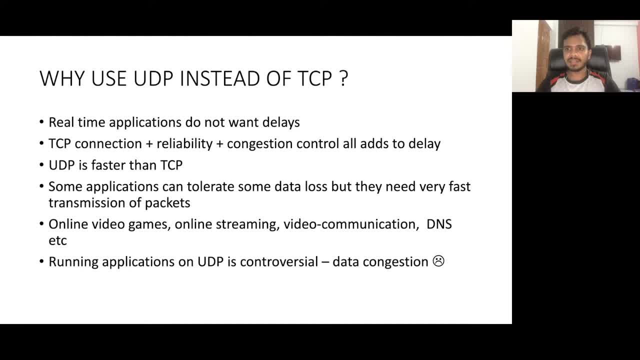 i mean like whenever you uh load a website, there will be slight delay, like slight more delay than when you use udp for dns. so that's why uh sometimes using udp is useful and also running applications on udp is controversial. the reason is that see one of the 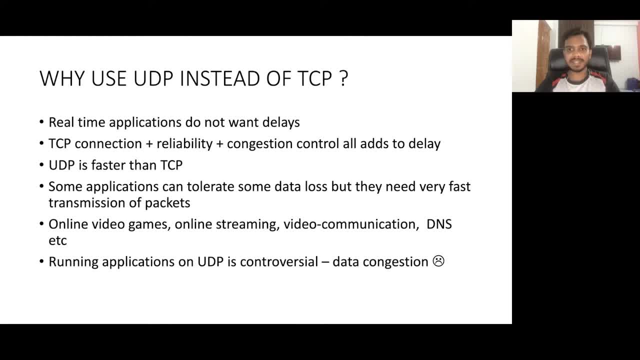 advantages of using tcp is like it also helps in congestion control. so what is congestion control here? is that so let's say, if the overall network, so the overall internet we have, if it becomes congested, then tcp protocol will help in that, like help in decongesting that network. but udp. 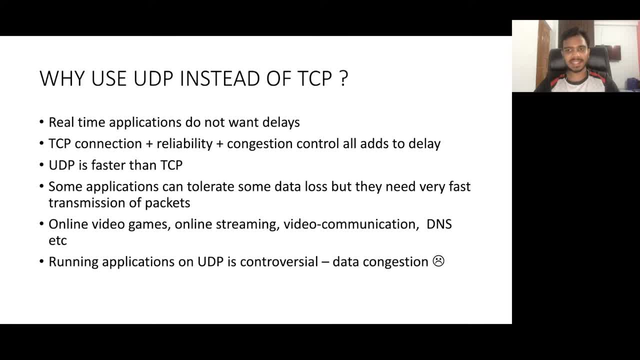 will not help, because udp only does demultiplexing and multiplexing plus some error detection, nothing else. so let's say if the overall network, overall network is over. so what do i mean by that? you know that overall network is congested. that means some of the routers are very busy, like they're getting 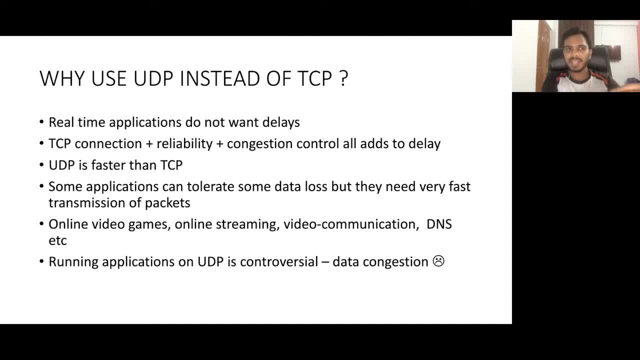 a lot of requests and when your request goes to that router, it will take a lot of time, i mean, and sometimes your request may even get dropped from that router. okay, in term, and when there is very- uh, when there is a lot of congestion in the network, now udp, what will happen? udp does not care about. 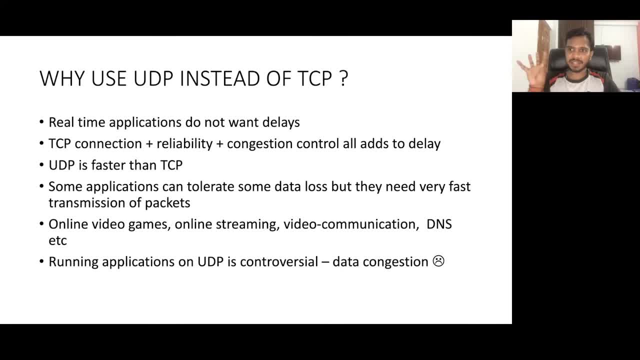 what's happening in network. so if you tell udp that, okay, i want to send this much amount of data, it will send it directly. it does not care about what is happening in the network. so of course, your network is already congested and you are sending more and more data in the network. so what will? 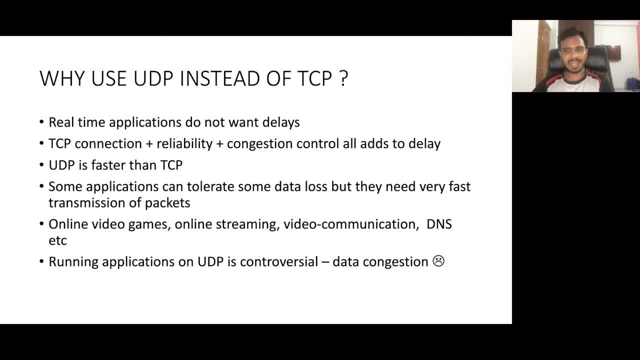 happen, the overall network will become more and more congested and basically there will be more and more packet drops and of course the users will see the issues. but in case of tcp this will be different. in tcp pc protocol we see that, okay, the overall- uh like network is congested, so it will. 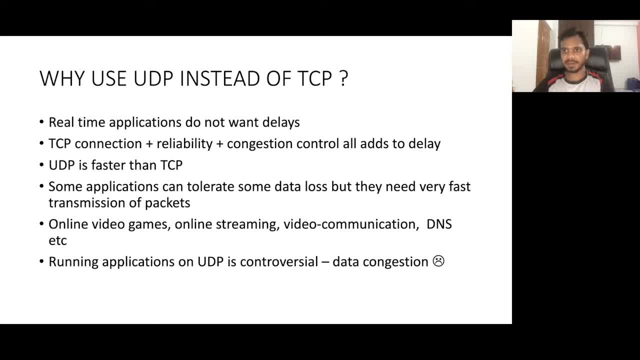 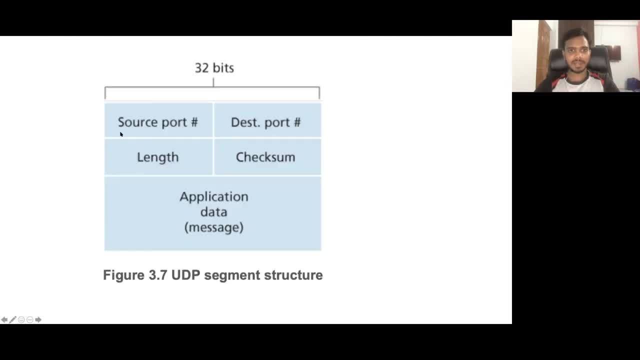 try to- i mean limit the uh transfer of data, uh from your system. so it will slow it down, so it will adjust it. now let's look at the overall network. so if you look at the overall network, at the udp segment structure, so if you see uh like in the headers or header of the transport layer, 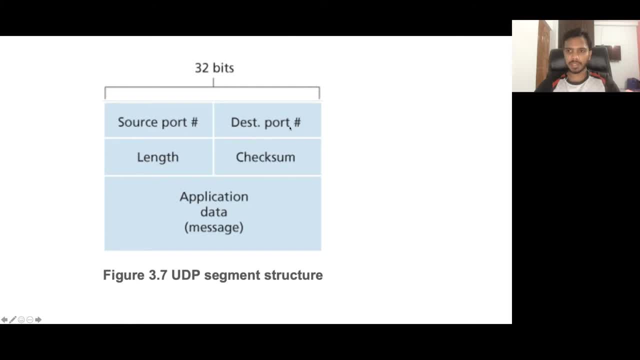 you have source port and destination port and this is very important and we have seen in the previous video in multiplexing and de-multiplexing how source port and destination port are very important, like they help in uh delivering the uh, whatever data, like the application is sending. 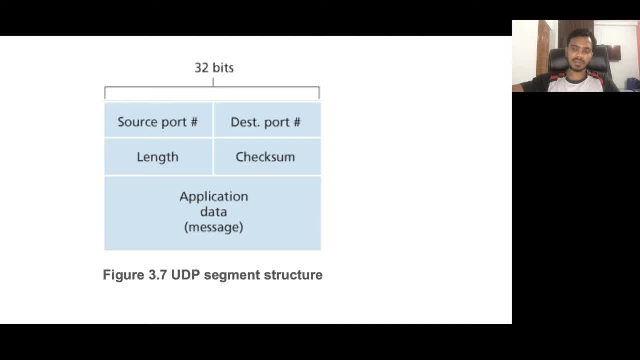 like it helps in sending that data to the correct process, right, because what will happen on server or or on your destination? there will be multiple process running and each process will be running on different ports. okay, so these ports help in differentiating between those process. so that's why i mean this source port and decision decision port are a part. 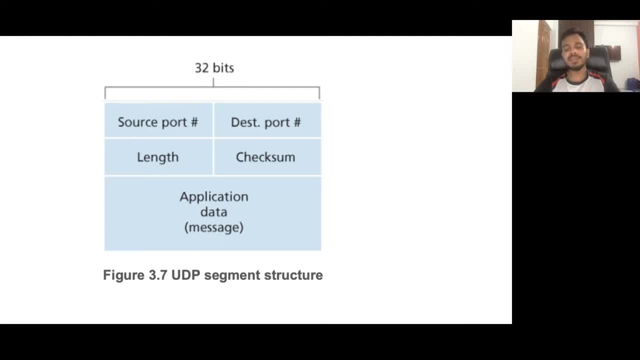 of transport layer and this will also be there in the uh when we see the tcp in the next video. so the source code is the board will also be there in the tcp segment. structure and, of course, length is there. what is the length of uh, this segment? then you have checksum, like checksum is used for. 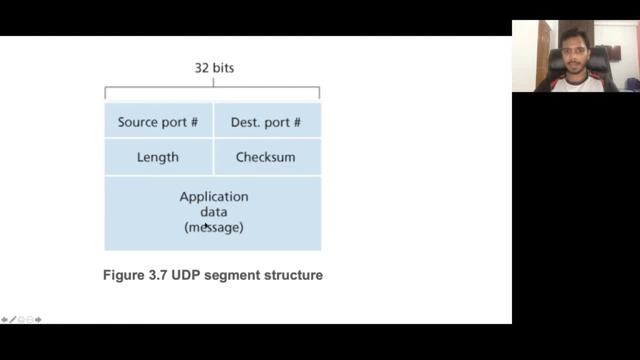 error detection that i have discussed above. and last one is, of course, the application data like message. so whatever application message is there. so basic transport layer function is to deliver this message like from, like uh, one process to another process, from source process to registration process. if you look at the udp segment structures, it's quite simple. if you see the most most. 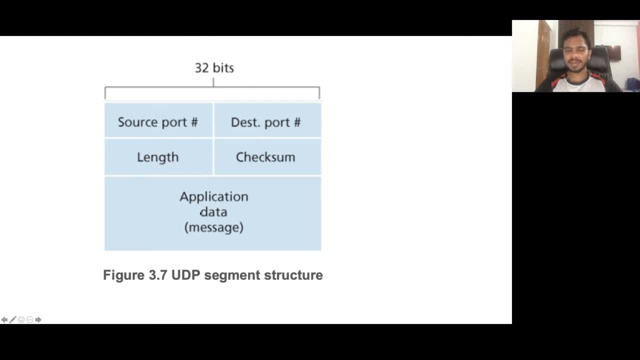 important ones are the source for decision port and of course then you have data. but as you will see, in our tcp segment structure it's a bit more complex than this because, again, because tcp is connection oriented, so it does have to store a lot of more information in the headers here. so next, 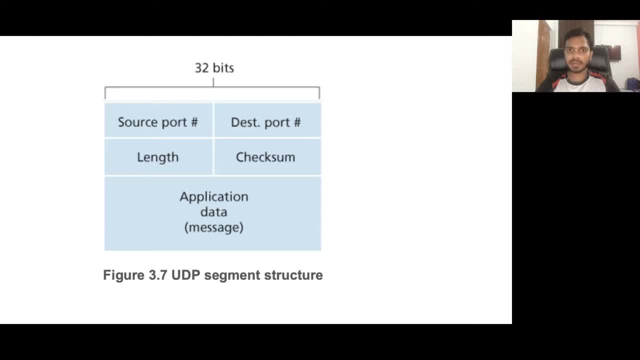 i will do is i will take an example, so, with the help of wireshark, to show you right how actually- sorry, how actually the udp communication takes place. and i will also show you this udp segment structure in that wireshark, because it's always better to again look at the real examples etc. 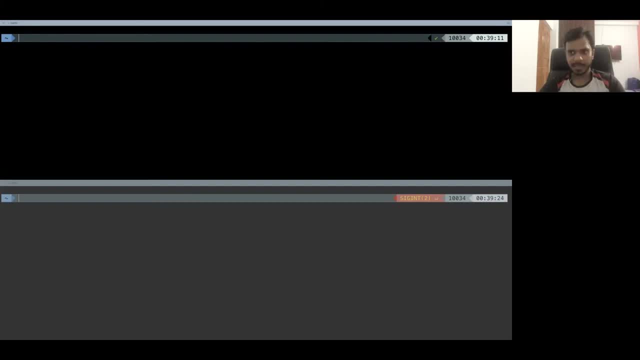 now for showing the example of udp protocol, a segment structure, with the help of wireshark. what i will do is i will use the ansi command or netcat command. so i have already made a video on ansi or and you can watch it. i will also paste the link of that in the description here. 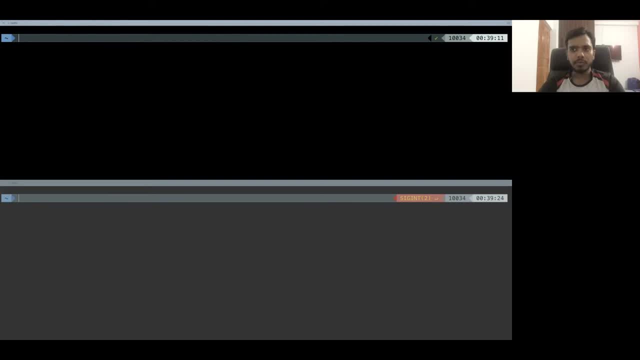 and what does command does is basically, it can be very helpful uh in in creating a very simple uh client server uh communication in order to create a very simple appliance server model communication. we can use that now. there are many other uses also of nc command and i've discussed 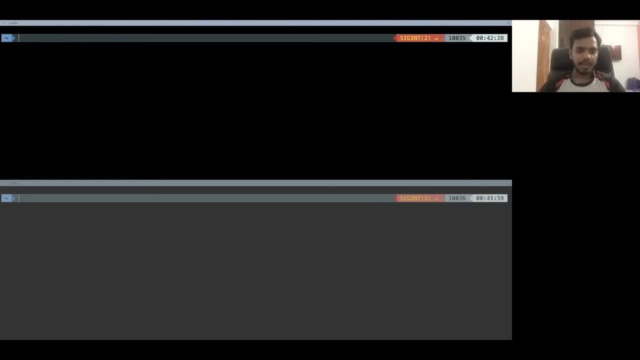 all of that in that video. so in the upper window what i will do, i will start the server here. so nc minus ul, so minus u. u flag is for udb protocol, l is for listening and basically i am starting the server on my localhost 127, 0.0.1, and i'm starting my server on port number one, two, three, four, five. 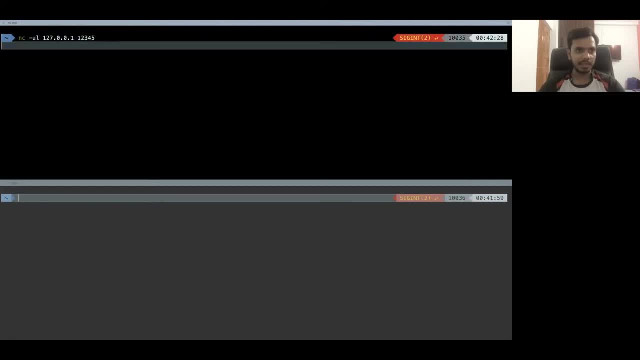 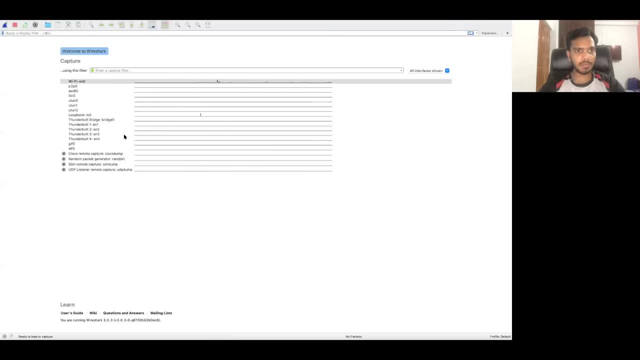 and i will start this. okay, now this. this has started. the- uh, the server has started. now i will go to the second tab and also, what i will do is one more thing: i will go to my wireshark here. okay, now, what i am doing. i am doing the communication on my local, local host network. 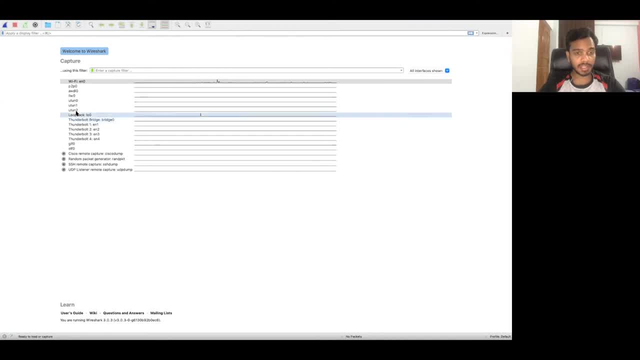 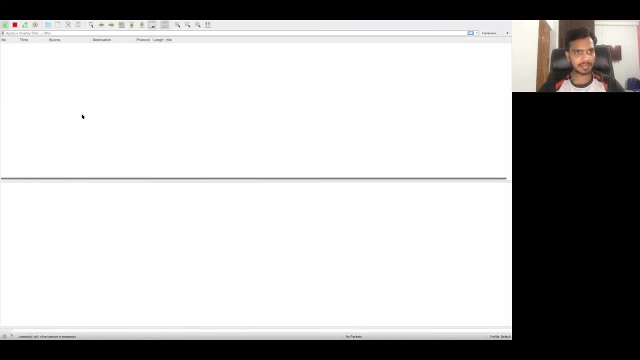 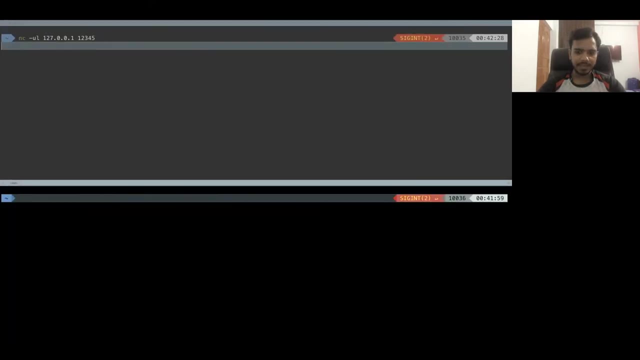 so for that i will select my local- hope, sorry, local interface. that is this one loopback. i mean, the local interface is also called as loopback, so i will select this. okay, now there are- uh, i mean there is nothing and no packets here. now i will go here and connect the client here, basically to. 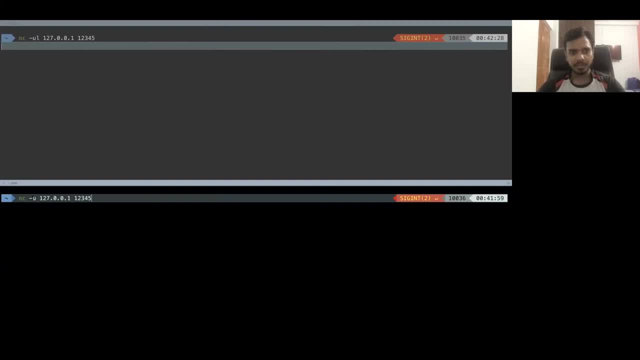 this server. basically, i will do uh nc minus u. u is for again udp, because i want to communicate over ud protocol and again i want to uh connect to the server which is there on this host 127, 0.0.1. that's why this and on which port the uh server is there? right one, two, three. 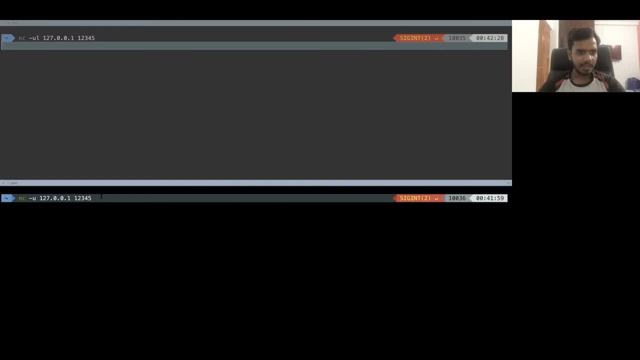 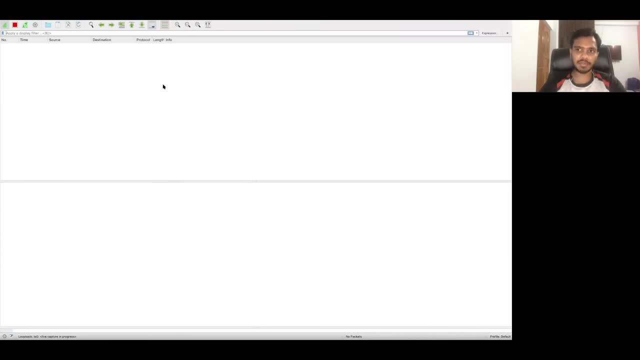 four, five. i will use that now. this is our client in the second one. i will press enter. okay, now let's go to this wireshark you. till now you see nothing right because, as i have told you, udp is a connection uh list protocol, so there is no connection happening here. that's why you are. 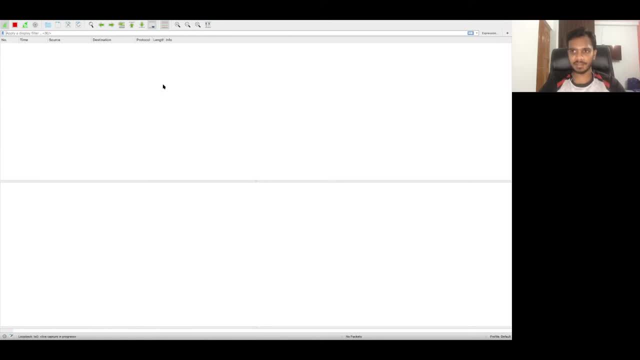 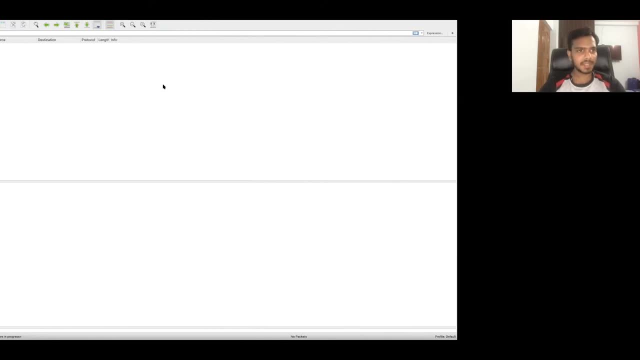 not seeing anything here. in tcp you will see it differently. do do note this in tcp also. i will show you the same example using as you can see in tcp. also, i will show you the same example using nc command, but you will notice some difference there. now what i will do is i will just say hello. 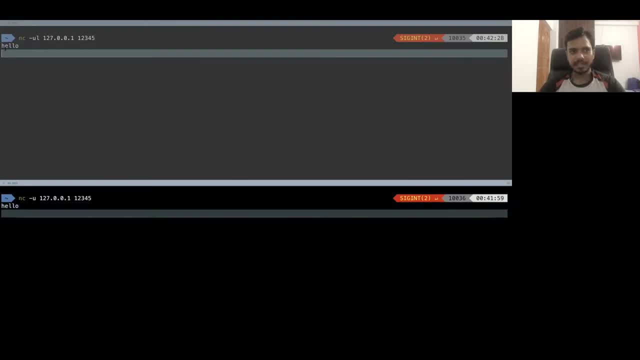 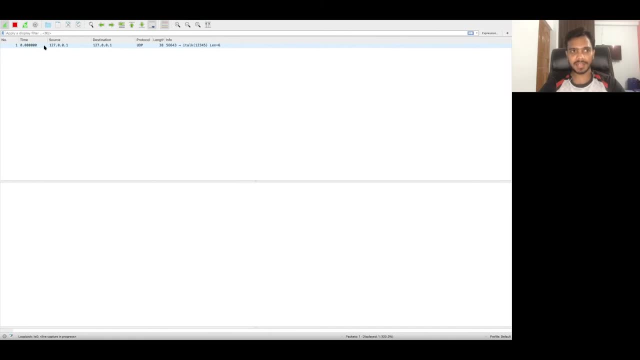 from client. so what you will see when i say hello, of course in the server also, you should see the hello here. okay, now let's go to wires, a wireshark. of course you see one uh frame here, right, let's click on this. okay, now of course, the first. i mean we have the four, uh, four layers here, right, the. 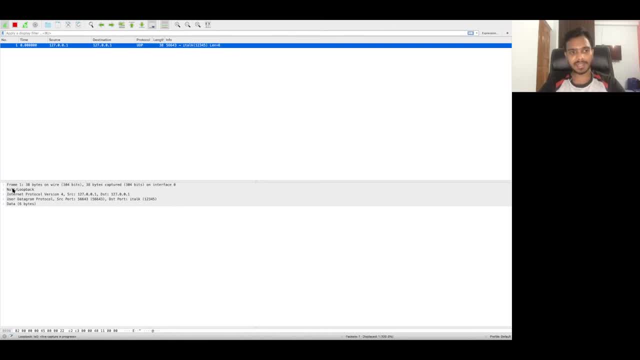 second: of course this is the frame. then you have the uh data link layer, but of course there is null back, because here we are just using a local host, so there will be not much information here. so there's no much information here now. also, we are not caring much about the data link layer here. 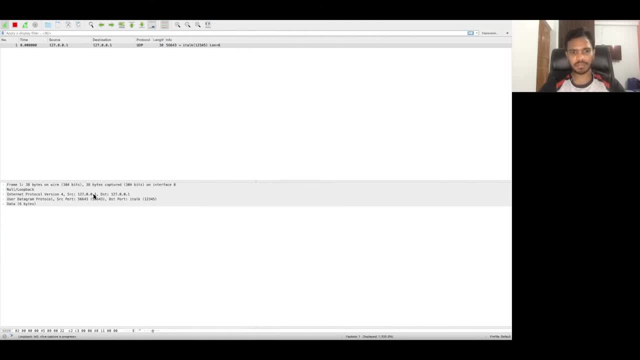 we are mostly if you look at the ipv4 address, of course. so the destination address is same, because i am communicating from 127 0.0.1 to 127 0.0.1. that's why both are same. but how we can. 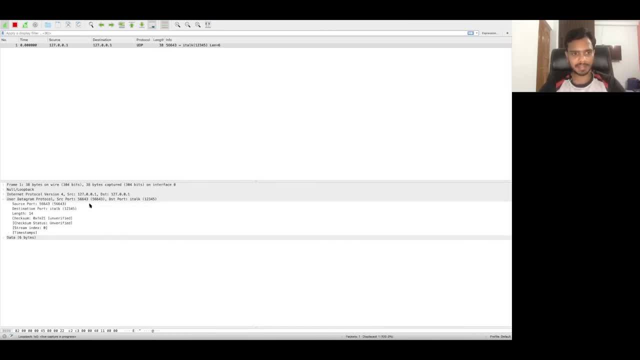 differentiate it. see the port number. the port number will be different. so you see here, the uh destination port number is one, two, three, four, five, because client is sending the message to server. that's why the the destination port is one, two, three, four, five, because destination is the server. 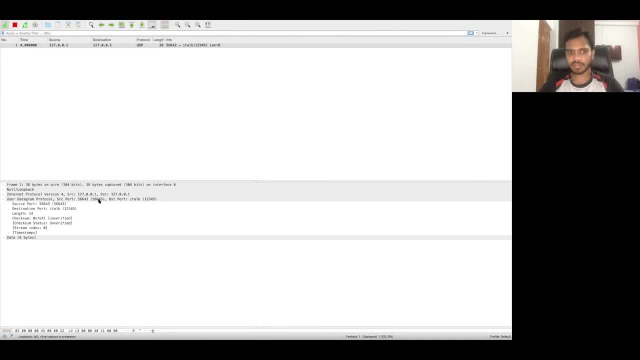 here and the client- the client- has started its socket. the client socket is running on this port: number five, six, six, four, three. that's why this is the source port and you can see right. source port is this and you can see some more information. i told you right, as you have seen here. source. 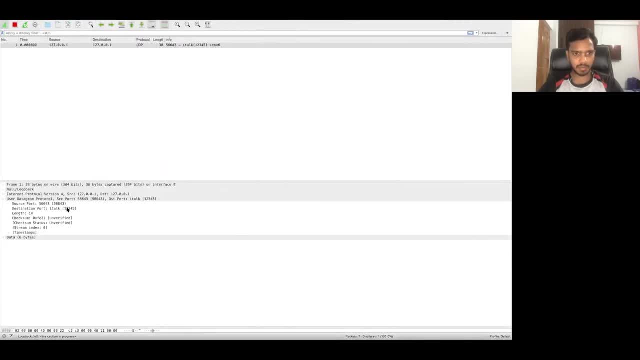 partition port is there, right, and you can see it's source code, decision port, and also there are names given for this. but of course you, you can see that at the numbers here: one, two, three, four, five and five, six, six, four, three. now, of course, length is there, okay, you see. 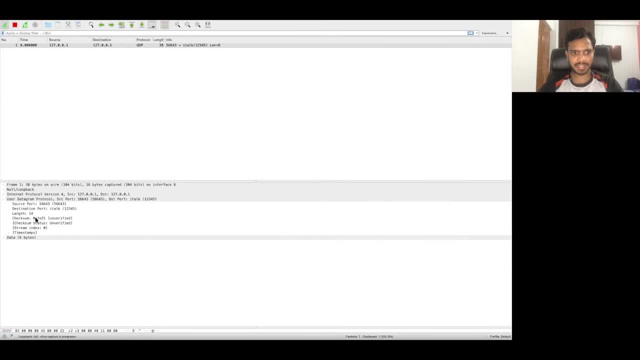 length here also 14 right, and there is some checksum for this. that is uh. i think that is in hexadecimal here. some checksum is also here. so these are some of the important uh fields in the udp, uh, udp segment, of course, and also you can see our data, so data is basically part of so, of course. 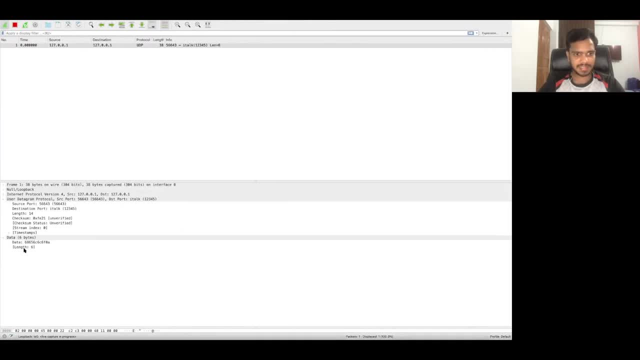 you see here, application data should also be there, right, and of course, data is there. that is of six byte and data is basically kind of: uh, it is not in the same format. if you click on this, okay now, if you click on the data, you can see, right, what we have sent. hello, because there is no. 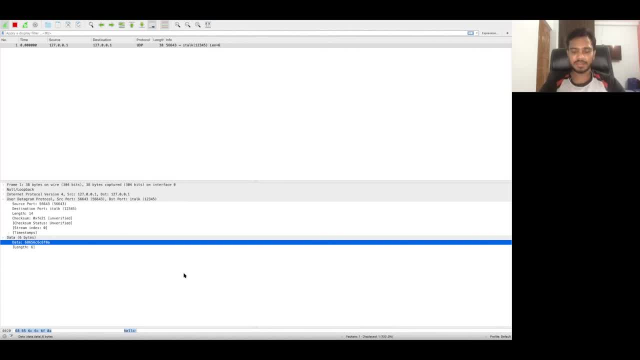 encryption that i have used here. right, i have sent the same hello message, so it's really visible on the wireshark. that's why you see hello here, right? so that's the communication ud protocol, and it's a very simple one, okay, one thing more i can show you. so of course, we know that, using the nc command, the. 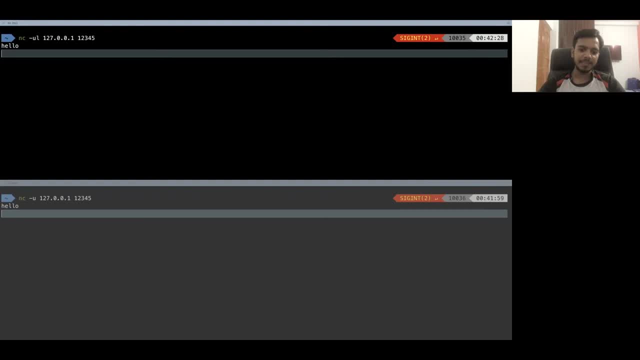 server can also communicate with the client. so if you type something here, let's type hello from server, okay, so of course you should see the reply, the same thing in the client also. you see the client. you see hello from server. this is our server side. now let's go to this wireshark you. 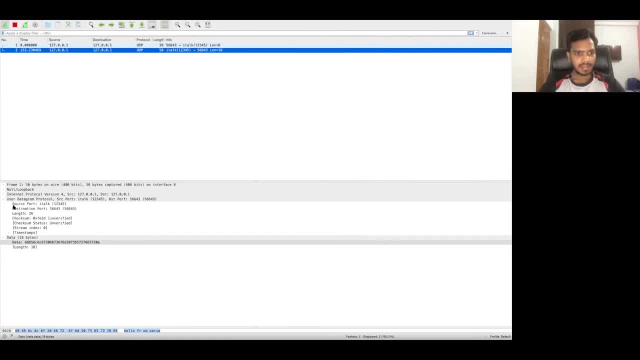 should see a second frame also here. let's click on this. but in this case again, if you go to uh, like the network layer, that is ip protocol here or network layer protocol, source solution is same. but of course, if you see UDP information, of course you see the source and destination port has reversed now. 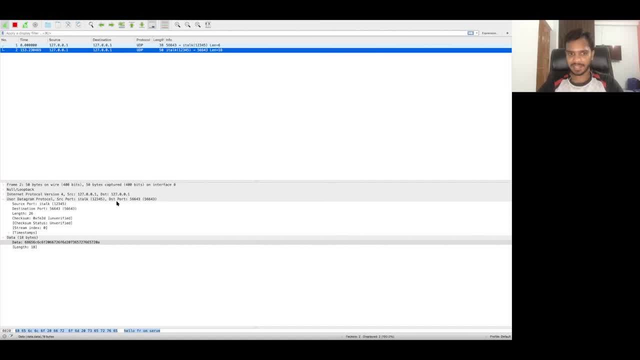 So source port is basically the server port 12345 and destination port is 56643. that is the client and not the socket on which client is running. Similarly, you can see source port: destination port length is 26 because here I have typed hello server right, hello from server. okay. 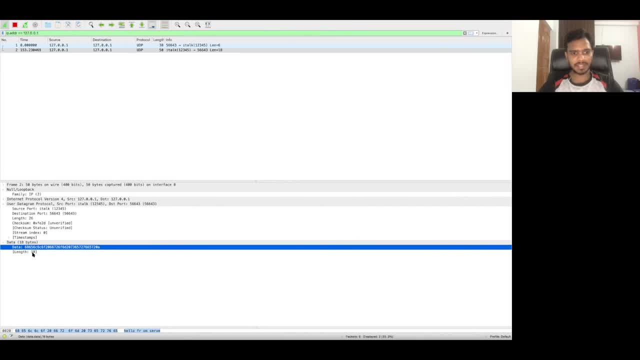 And also you can click on the data itself. the length of this is 18.. So length of this is 18 and overall length of like this segment is 26, and also you can see the data here. hello from server. you will see in this data here. 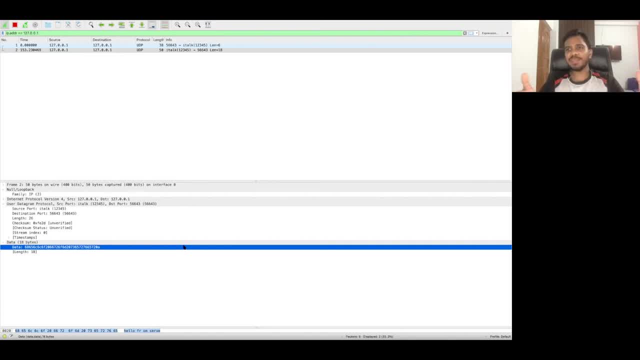 So that is simple example of communication using UDP protocol. and you see, UDP is quite simple. if you see, even the segment is quite simple, like you see only source, port, destination, port length and checksum, and if you see the communication, it's quite simple, right you? 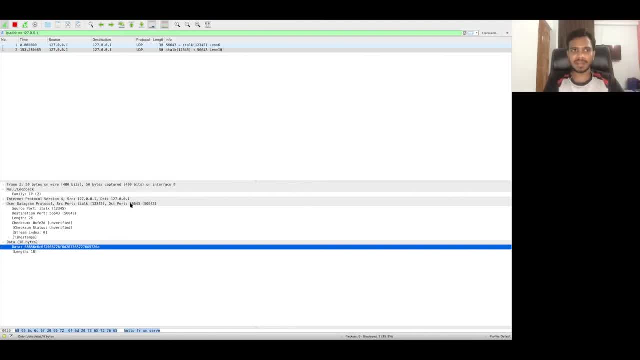 just, I mean you send like it. yeah, if the data is big, what will happen? I mean the whole data will get break. I mean broken down into smaller, smaller segment. So that also example we will see later on. I am not going to show that example now, but 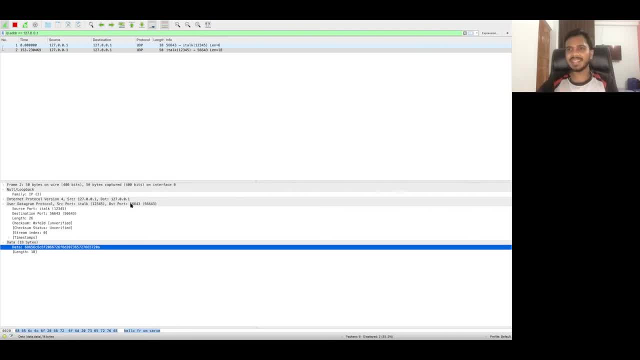 yeah, we will take one example where the data size is very big. here the data size is very small. right, hello from server or hello. So in just the, in just one frame or in just one segment, the overall data is sent, right. but when you have a very big data in that, what can happen? the whole data will not fit.